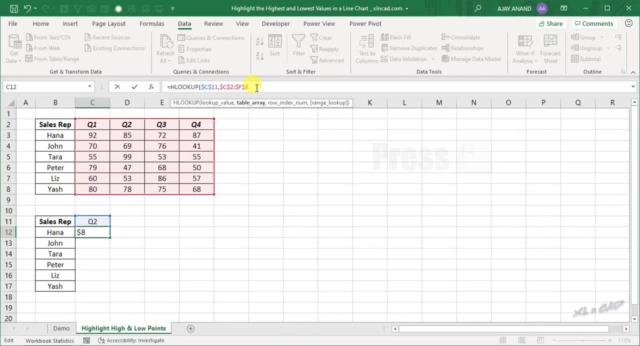 make the cell reference absolute. comma. row index number. we'll use rows function here. open parenthesis. select the cells c2 to c3. we'll make the cell reference c2 absolute. close parenthesis. once again close parenthesis and press the enter key function. return the value 85, which is the sales figure of hana for the second quarter. copy the: 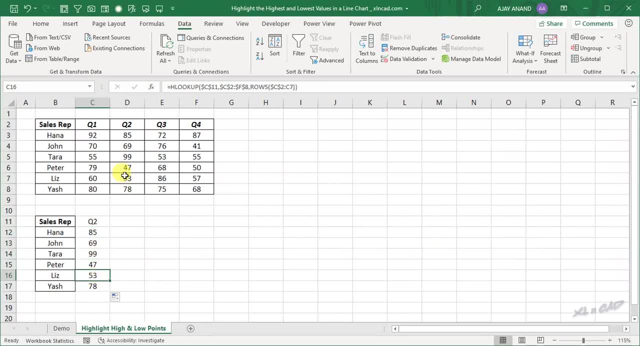 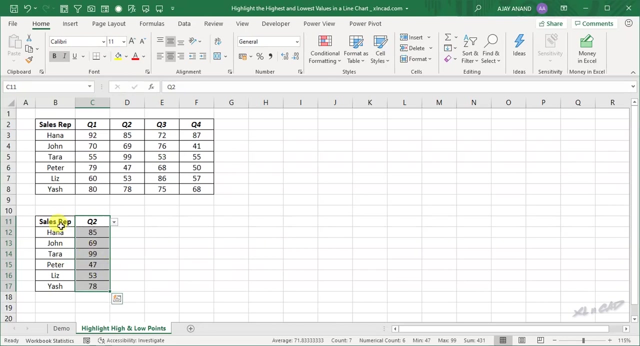 form line to the downward cells and we have the entire sales figures for the second quarter. we'll change the quarter from this drop down menu and we will have the sales figures for the corresponding quarter. we'll apply the same formatting: home tab format painter. now to create a line chart using this data. select the data, go to the insert tab, insert line already. 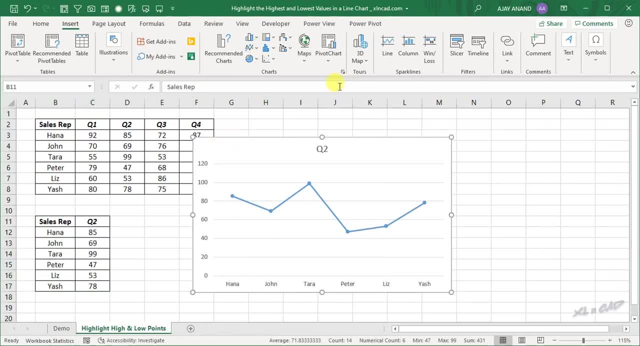 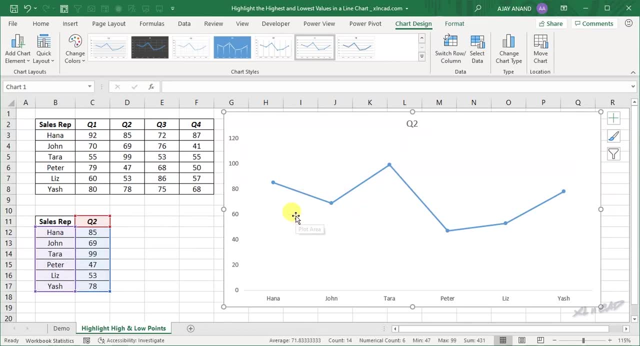 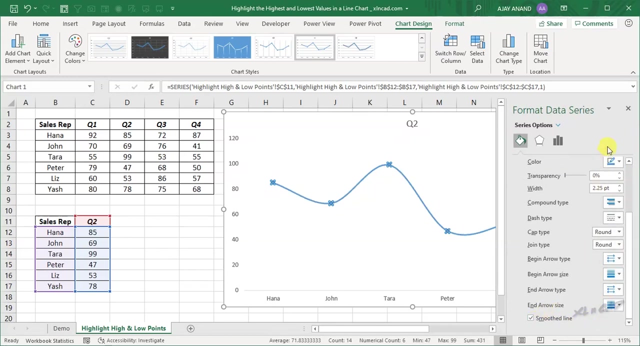 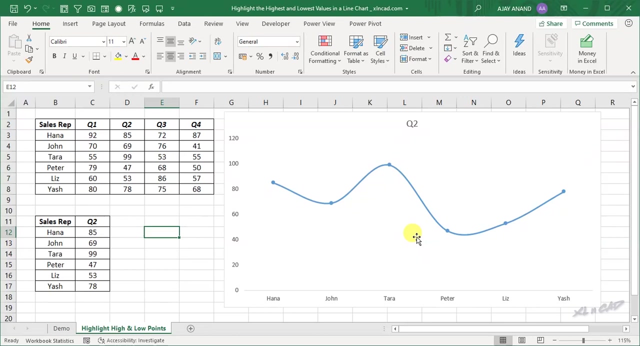 chart line with markers will resize this chart. will delete the grid lines. to smoothen this line, right click on this line. format data series, fill in line, scroll down. mark the checkbox for smooth line. now about highlighting the high and low points of this chart. for the same, we will be using separate data series to 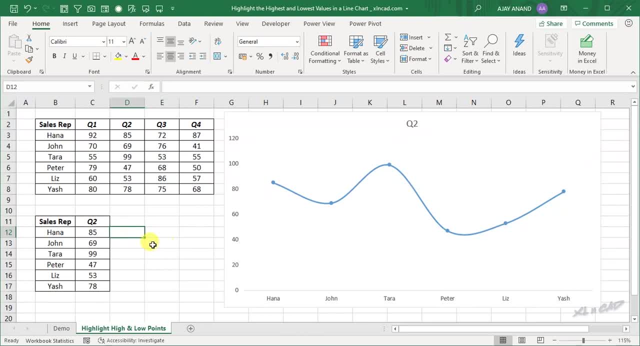 create a data series for the high point. select this cell in the formula bar: equal if function. open parenthesis. select the cell setol: equal max function. open parenthesis. select the cells from setol to c17. make the cell references absolute: close parenthesis. using this logical test here we are checking whether the value in the 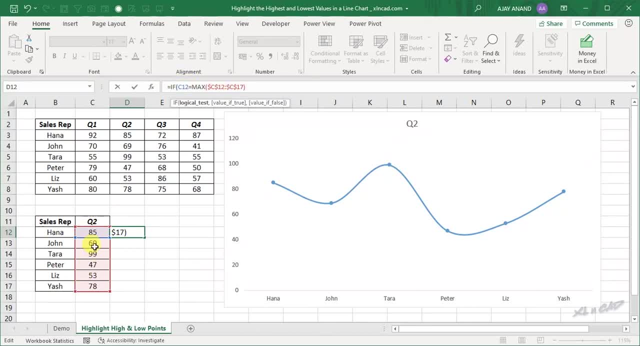 cell setol is equal to the largest value in this data range. comma value. if true, the value to return when this logical test is evaluated as true. if the value in the cell setol is equal to the largest value in this data range, the function should return the value in the cell setol for that select. 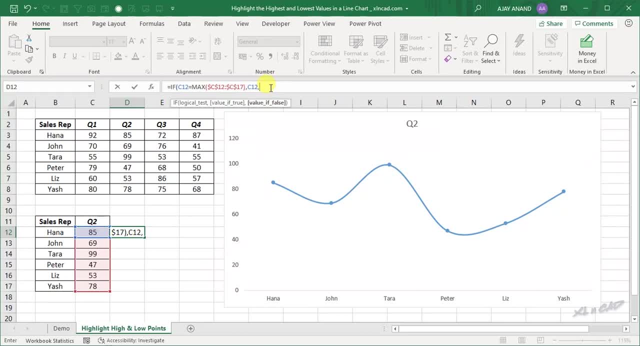 the cell setol and click OK. setol- comma value: false. if the logical test is evaluated as false, function should return a not available error. Na open, close parenthesis and once again close parenthesis and press the enter key. function has returned a not available error. so we have copied the former line to the downward cells and we have the largest value in the. 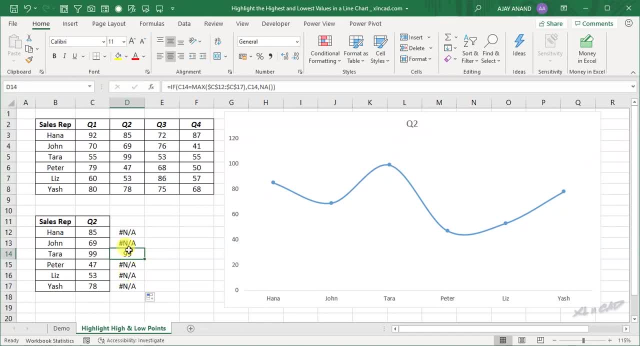 cell setol range beyond and the expression the largest value in this data range to plot the data throws into the tots here. it's very simple, does not arrested this also short this line chart. right click on the chart, select data. add series values. select the data series will name this series as max. 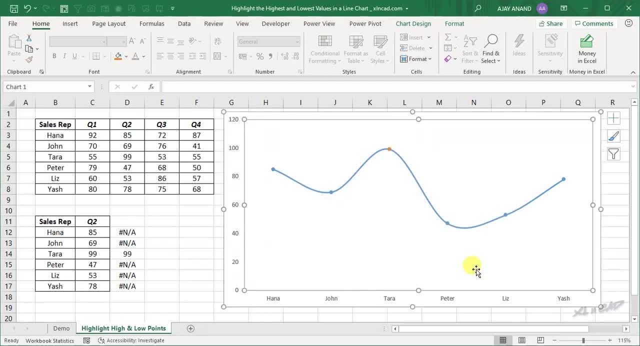 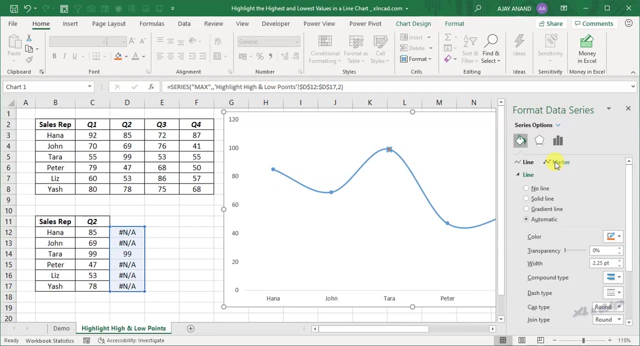 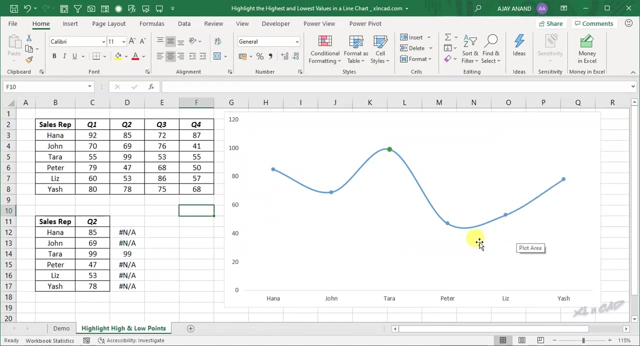 okay, once again okay. and here we have the high point in this chart. to format this marker, right-click format data series fill in line marker marker options built-in. will increase the size to 7. to change the color fill will make it green in the same manner. 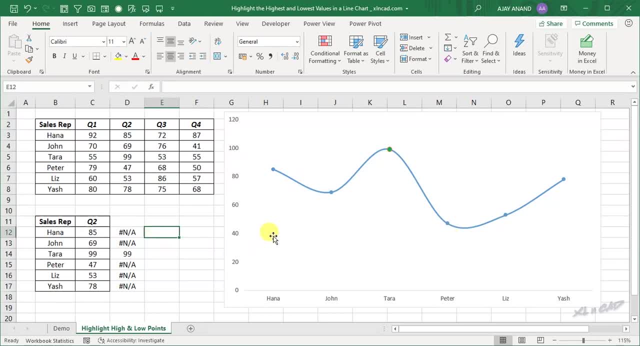 to plot the low point. select the cell equal if function. open variances: select the cell ctool equal. main function: open variances: select the cells from ctool to c17. make the cell references absolute. close variances: comma: select the cell ctool comma in a function. 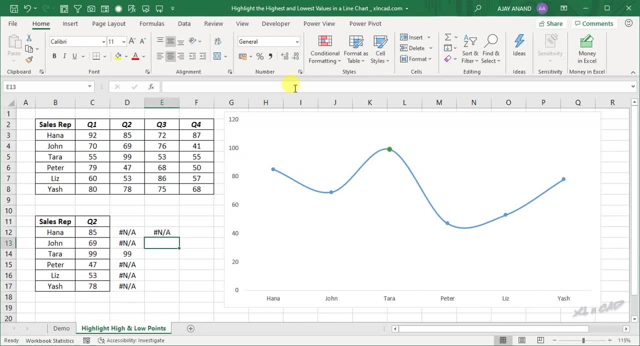 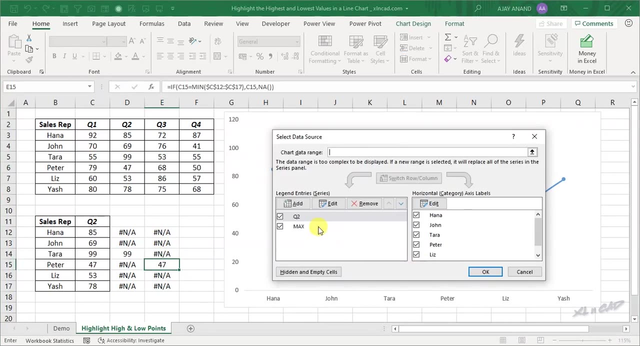 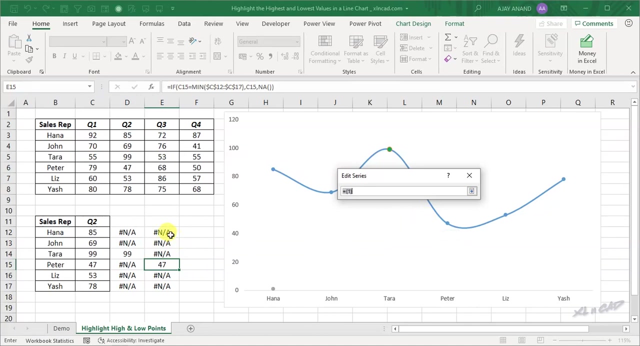 close variances and press the enter key. copy the formula into the downward cells. here is the smallest value in this data range. to plot this data series into this chart, right click select data add will name the series as min series values. select the data series. okay, once again, okay.